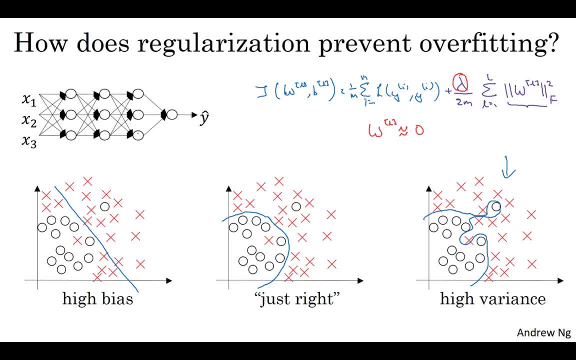 So one piece of intuition is: maybe it'll set the weight to be so close to zero for a lot of hidden units that it's basically zeroing out a lot of the impact of these hidden units. And if that's the case, then you know. 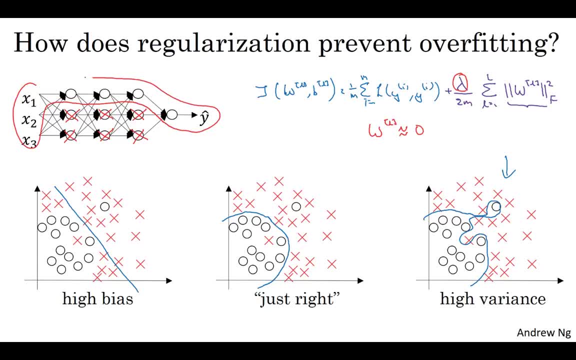 this much simplified neural network becomes a much smaller neural network. In fact, it's almost like a logistic regression unit, you know, but stacked multiple layers deep, And so that will take you from this overfitting case much closer to the left, toward the high bias case. 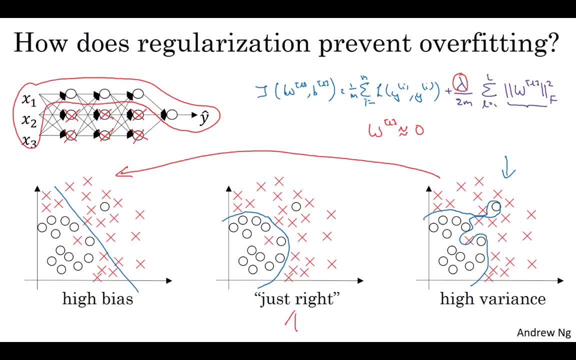 But hopefully there'll be an intermediate value of lambda that results in a result closer to this, just right case in the middle. But the intuition is that by cranking up lambda to be really big it'll set W close to zero, which in practice this isn't actually what happens. 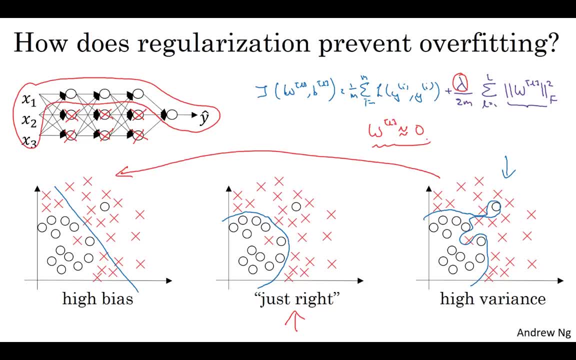 We can think of it as zeroing out or at least reducing the impact of a lot of hidden units. So you end up with what might feel like a simpler network that gets closer and closer, so as if you were just using logistic regression, The intuition of 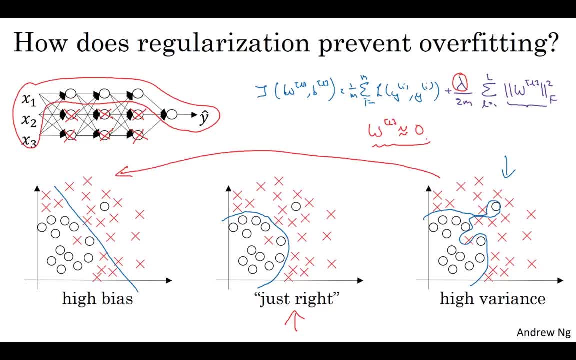 of completely zeroing out a bunch of hidden units isn't quite right. It turns out that what actually happens is it'll still use all the hidden units, but each of them will just have a much smaller effect. But you do end up with a simpler network and as if you have. 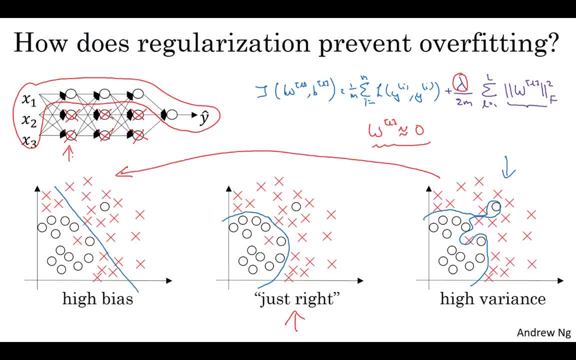 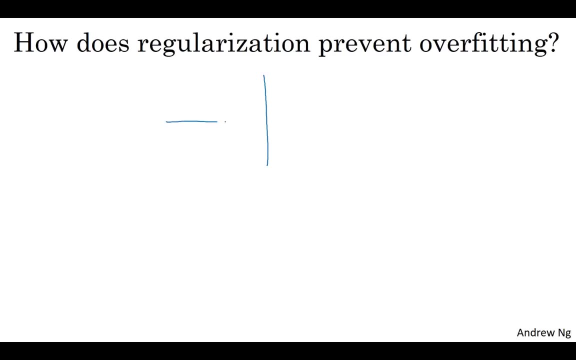 a smaller network that is therefore less prone to overfitting. So I'm not sure if this intuition helps, but when you implement regularization in the programming exercise, you actually see some of these variance reduction results yourself. Here's another attempt at additional intuition for why regularization helps prevent overfitting. 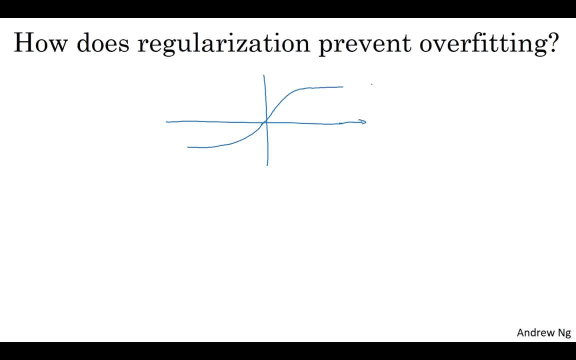 And for this I'm going to assume that we're using the tanh activation function, which looks like this, right? So this is: a g of z equals tanh of z. So if that's the case, notice that so long as z is quite small, 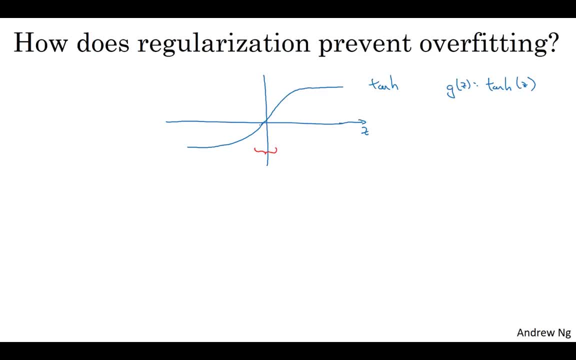 so if z takes on only a smallish range of parameters, maybe around here, then you're just using the linear regime Of the tanh function. It's only if z is allowed to wander out, you know, to larger values or smaller values, like so. 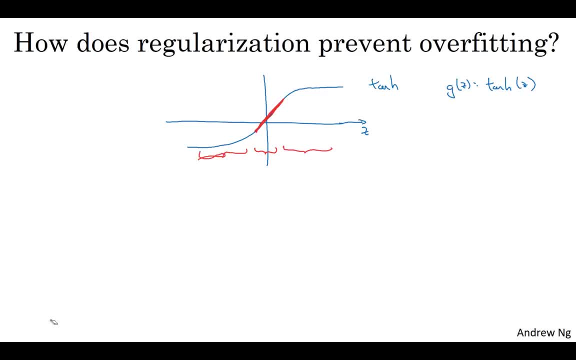 that the activation function starts to become less linear. So the intuition you might take away from this is that if lambda, the regularization parameter, is large, then you have that your parameters will be relatively small because they are penalized to being large in the cost function. 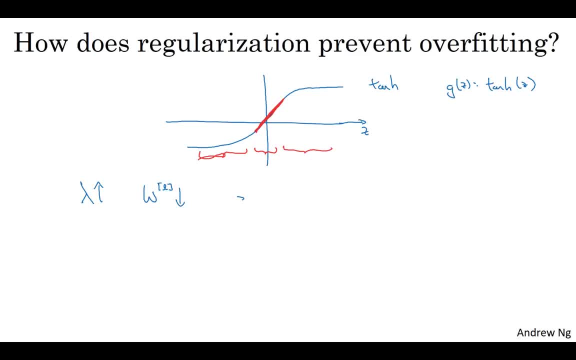 And so if the weights w are small, then because z is equal to 1, z is equal to w right and then technically it's plus b. But if w tends to be very small, then z will also be relatively small. 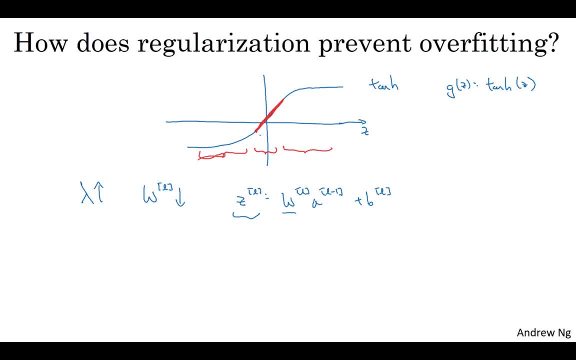 And in particular, if z ends up taking relatively small values just in this little range, then g of z will be roughly linear. So it's as if every layer will be roughly linear, as if it's just linear regression. And we saw in course one. 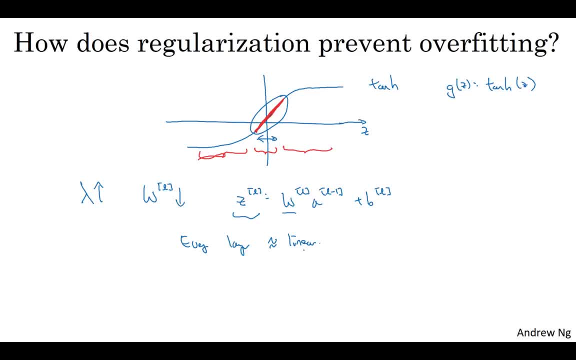 that if every layer is linear, then your whole network is just a linear network, And so even a very deep network with a deep network with a linear activation function is, at the end of the day, only able to compute a linear function. So it's not able to, you know. 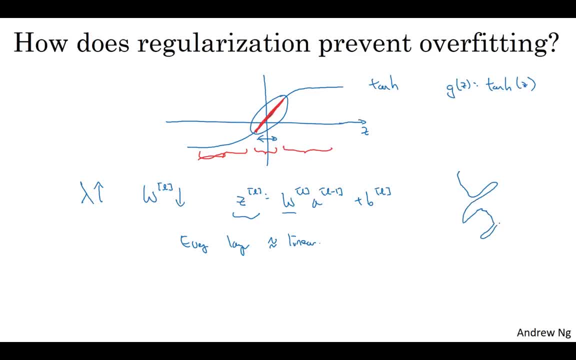 fit those very, very complicated decision, very non-linear decision boundaries that allow it to, you know, really, uh, overfit right the data sets, Like we saw on the overfitting high variance case, um on the 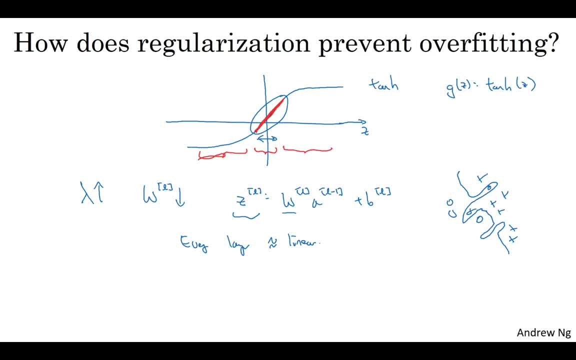 on the previous slide. okay, So just to summarize, um, if the regularization parameters are very large, the parameters w are very small, so z will be relatively small, kind of ignoring the effects of b for now, Um, but so z is relatively. 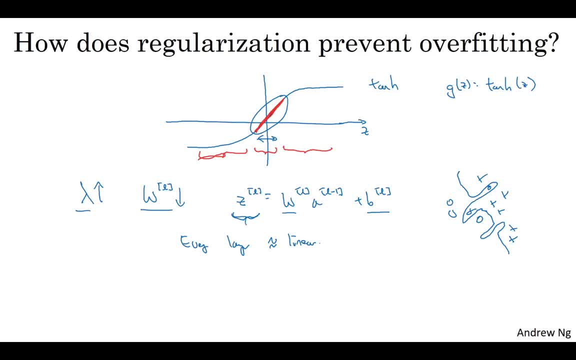 so z will be relatively small, or really you should say it takes on a small range of values, And so the activation function, if it's 10H, say, will be relatively linear, And so your whole neural network will be computing something not too far from. 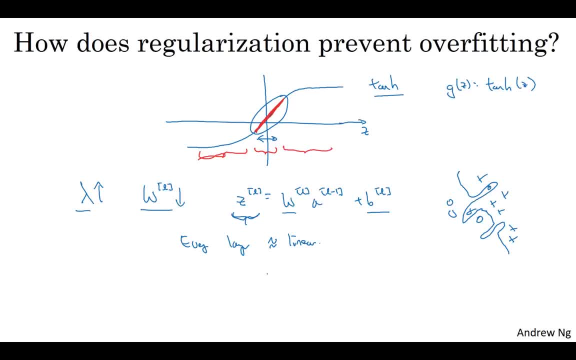 uh, a big linear function, which is therefore a pretty simple function rather than a very complex, highly non-linear function, And so it's also much less able to overfit. okay, And again, when you implement regularization for yourself in the current exercise.